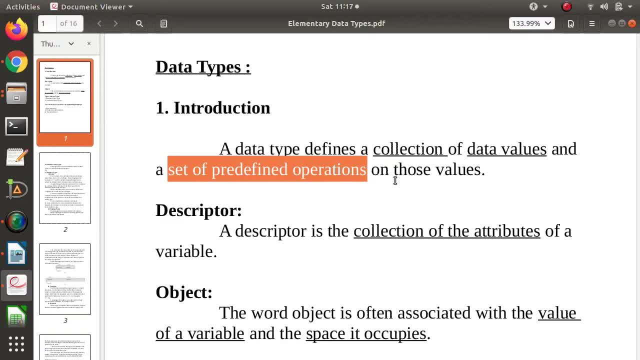 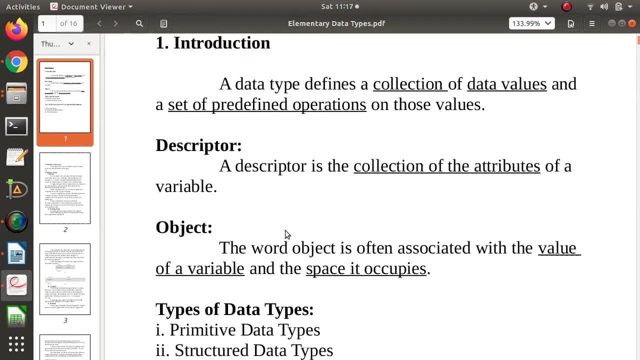 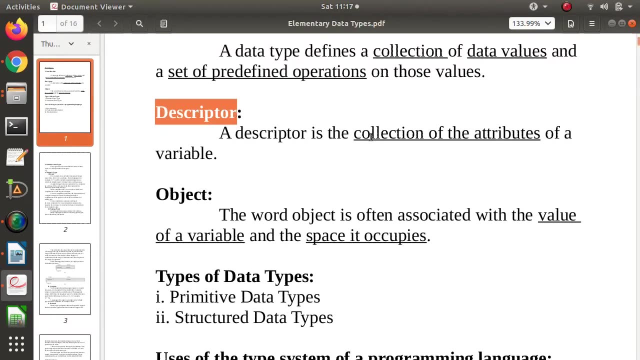 some operation on that. we can allocate some values to that. so values and predefined operation define a data type. now there are some uh terminology. those are used along with the data type. so one is descriptor. so descriptor means collection of all attributes. collection of all the attributes of a variable is called 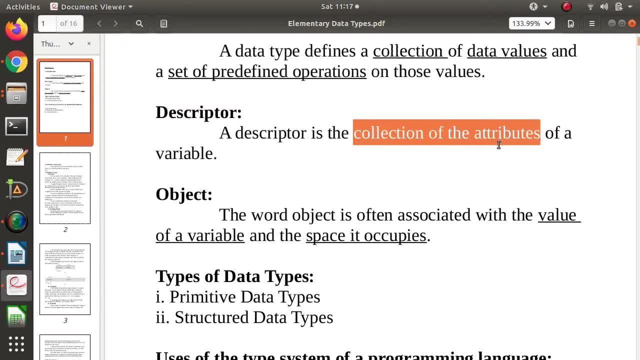 as a descriptor. now, what kind of attributes? so see, for every variable it has some name. so, for example, if we take integer x, so x is the name that we have given to that variable. so this is one attribute. then what is the data type? int- that is one attribute. then x will have. 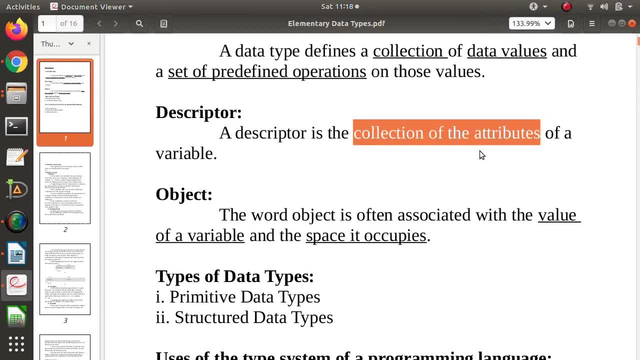 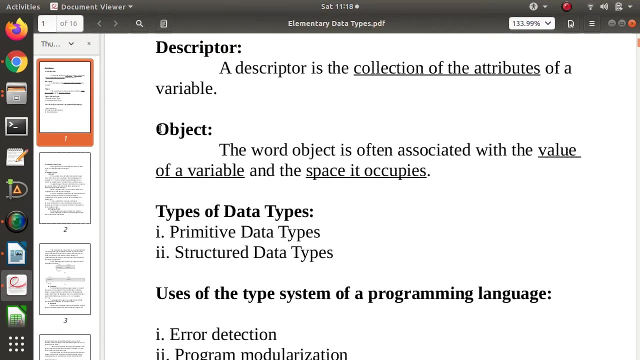 some value, so that value is also attribute. then, uh, some memories get allocated to that variable, that is also an attribute. then it will have some scope, that is also an attribute. so collection of all the attributes of variables, so that, uh, all the attributes together is called as a descriptor, then object. so one more terminology. 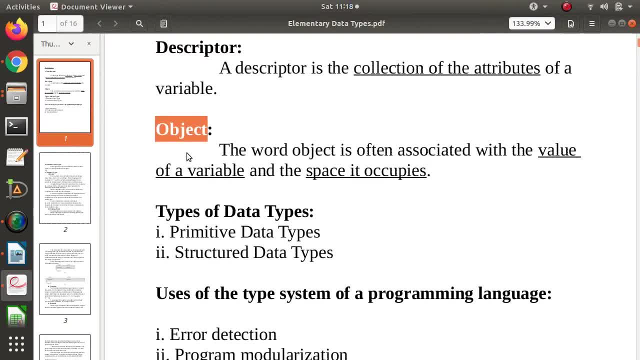 that is used with data type is object. so normally, uh, we use this terminology, uh, or this word, object for the instance of class. so normally we use for that purpose. so object is an instance of class. so basically, object is a variable of type, that particular class. so suppose, if you have a class, 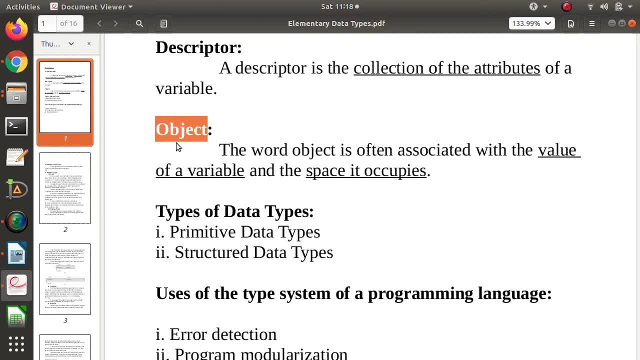 we are defining, suppose s1, object: student, s1, so s1 is a variable of type student. so in that way normally we use, but in broad sense object is also used to call any variable. so object means any variable. so how we can define object, so value of a variable and space it occupies. so for example: integer x. so whatever the value that is occupied, then you can define the value of the variable, then the variable with that defined component. therefore it you will get the value of the variable. where is the value of the variable δ, as i have already described here, when we provide an argument there. related to that we have different methods of defining variable and value. so in the previous Progress i have already discussed- and Integers are outside of terms which we can define classfor, but with competitors we can also define a following model where we define values. so what is the value of the variable? 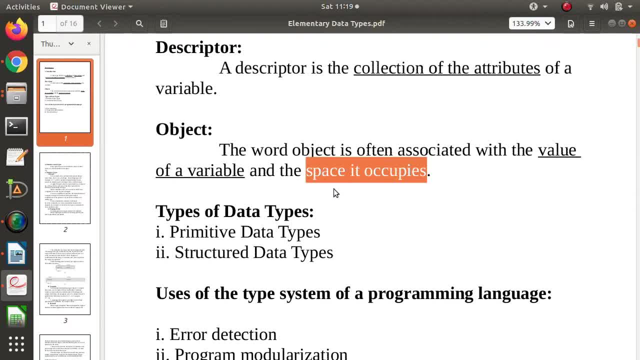 and which is equal to the number of applicants which we want to specify location and how that will check allocated to that variable and what are the memory that is allocated to that variable? So combinedly we call it object. So value along with address are what are the memory space that we are allocating to that? 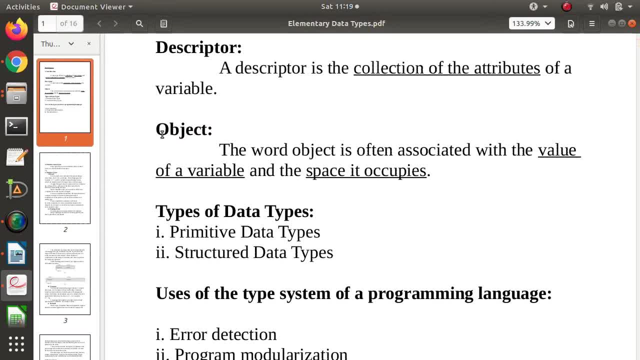 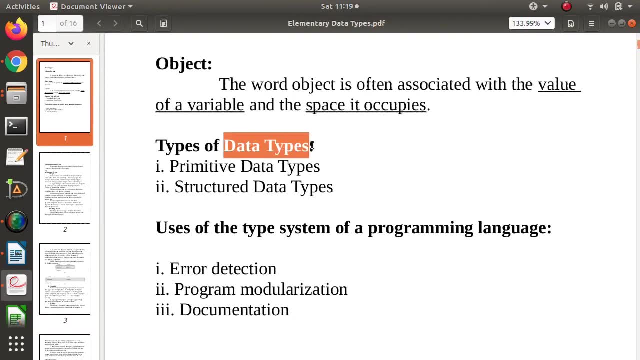 variable. So in normal sense we use object as an instance of class or variable of class. So in normal sense it is used for variables of all the data type. This is the object. Then there are different types of data types, So there are two types. 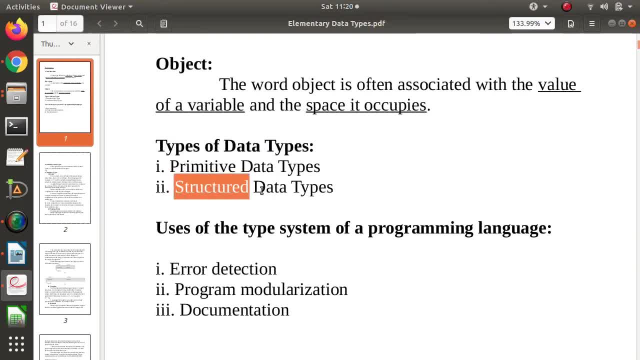 One is primitive data type and another is structured data type. Primitive data types are those types which are provided by any programming language or those are built in data types, or in other words, we can say data types which cannot be defined in terms of other data types. 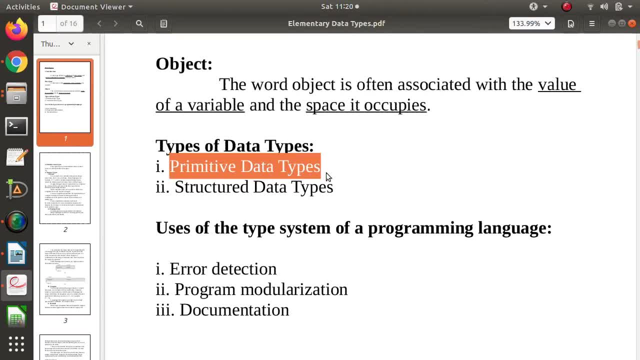 Those are called as primitive data types Or, in simple words, built in data types, For example, integer, float, character. all these are the data types which are provided by programming languages. So those are the primitive data types. So we will have next video based on these primitive data types. 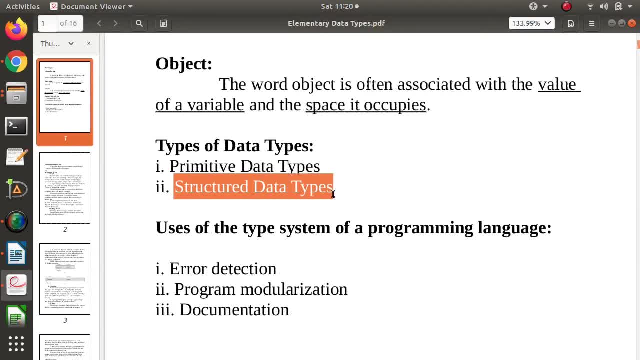 Then another type is structured data types. So structured data types are those data types which are defined from the other data types or from the built in data types, For example array. So array is a collection of other data types. Suppose, if we take array of integer, 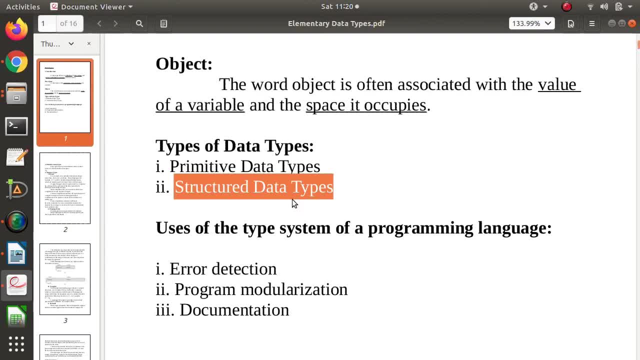 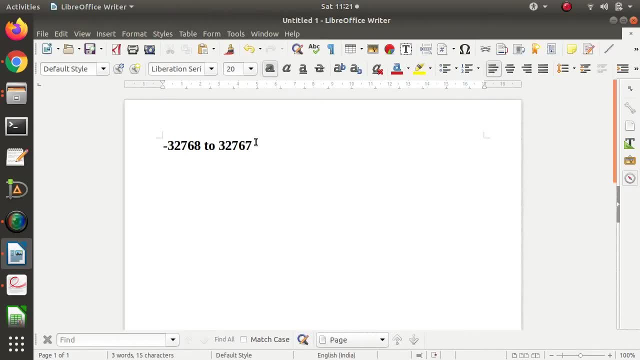 So array, that is the data type which is defined from the integer data type, Then linked list. So normally we define linked list in C language like this: So we define structure for that, Then some name, And in linked list we will have some value. 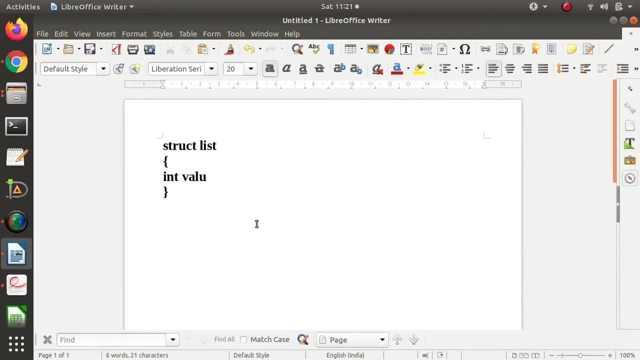 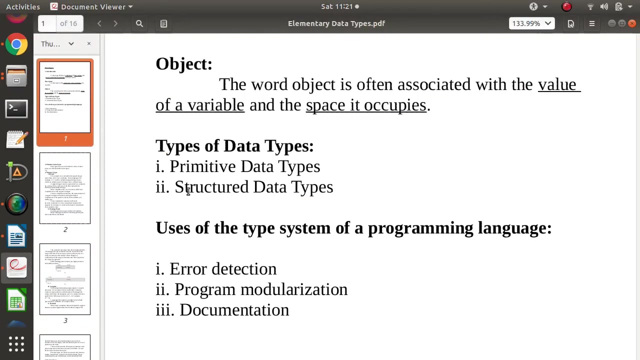 And it has some pointer Pointer to the next node. Now see, this is a structured data type, So which is defined in terms of other data types. Then we have classes, Classes, Classes, Records, Lists. All these are the structured data types. 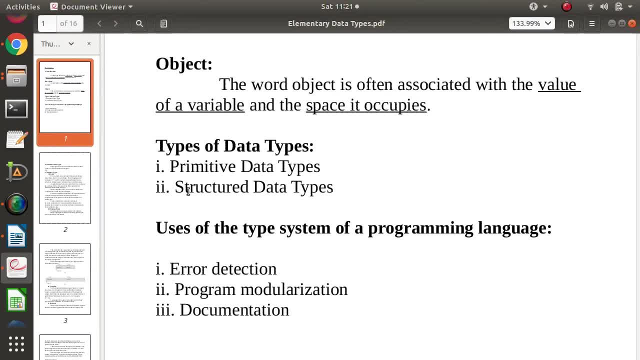 Data types which are defined in terms of built in data types or primitive data types. Those are called as a structured data type. So one terminology that is used along with the structured data type, that is abstract data type. So I have created some videos based on the abstract data types. 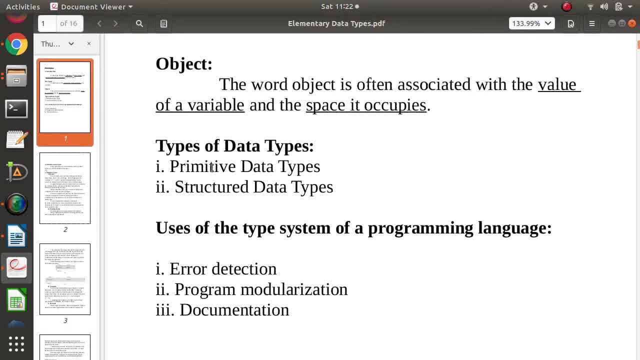 You can find it on my YouTube channel. So there are two types of data types. One is a primitive data type. Those are built in data types. Data types which are provided by the programming language or data types which cannot be defined in terms of other data types are called as a primitive data types. 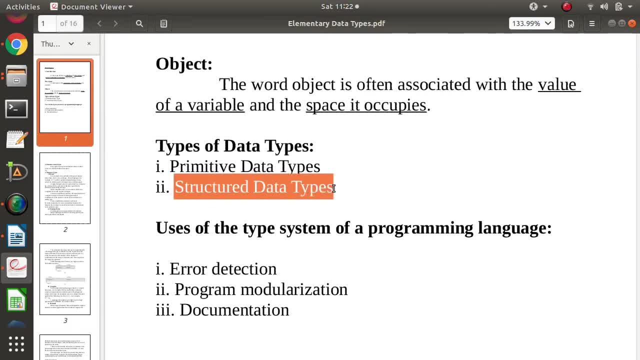 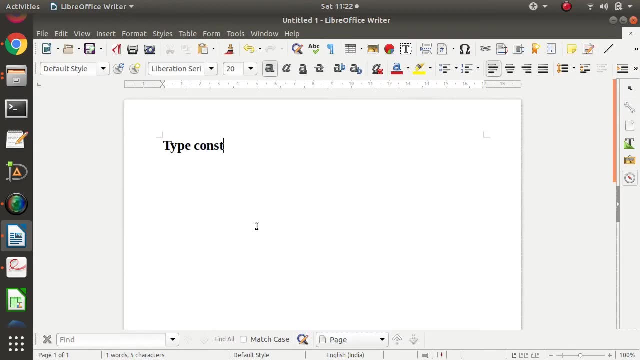 And structured data types are those data types which are defined from the primitive data types, And what are? the structure that is used to define this structured data type is called a type constructor- Type constructor, So it is a way to define Structured data type. 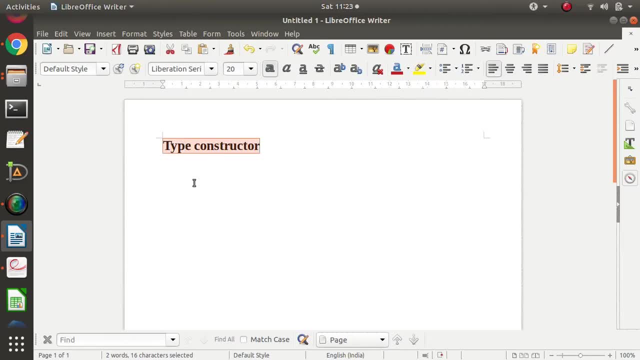 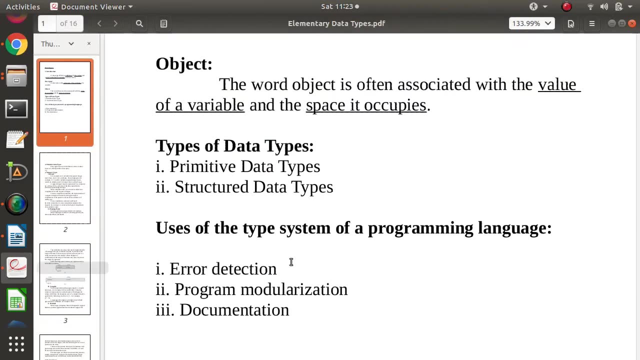 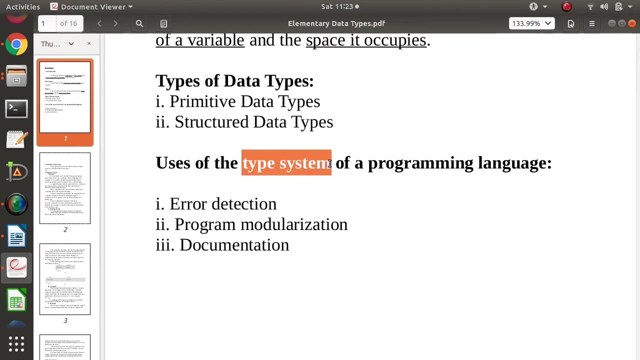 For example, we have seen definition of a linked list data type. So that is a type constructor for linked list data type. Now there are some advantages of type system. So basically type system of any programming language, in the sense all the data type, those 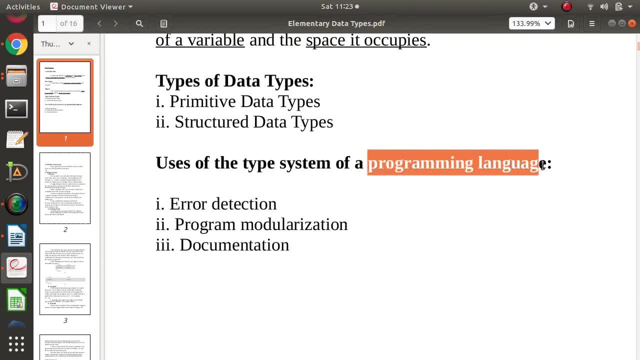 are provided by that programming language. So if you take example of C++ language, So type system of C++ language, you know all data types: integer, float character then, or some structured data type, for example array, structure, union classes. 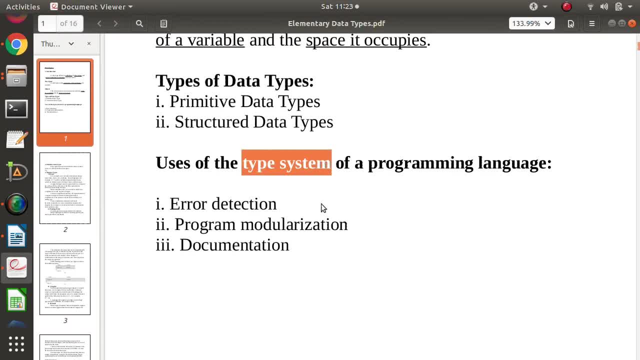 So that is a type system of C++ programming language. Now what are the advantages of type system of programming language? One is error detection. So whenever we are defining any data type, so it has some operations, it has some predefined operations Which we can perform on those variables. 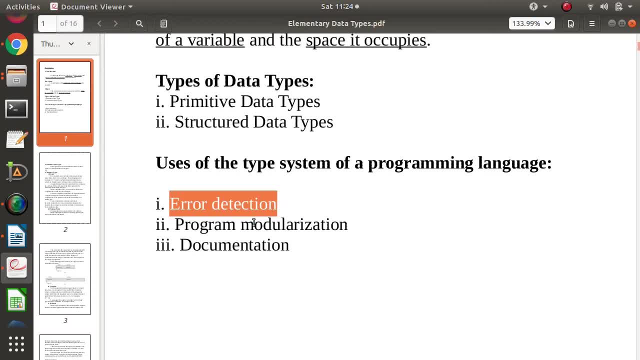 So if we are using for some different operations, so from there we'll get some error. And again, these data types can be used with the specific data types only. So, for example, we cannot use with the other data types or in any arithmetic expression. 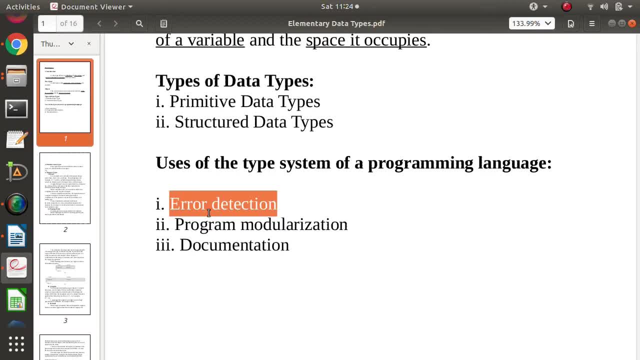 we cannot use data type with the other data types, a variable of one data type with the other data type. So there is a type costing. So those are the features provided by the programming language. But those are the different thing. But in that situation we can find out the error.